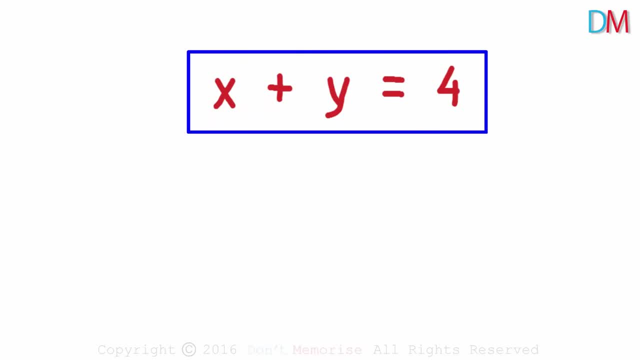 X and Y. Now how can this be represented on a graph? Let's have the coordinate plane on the right hand side. It's very easy to represent this equation graphically. All we need to do is find many pairs of X and Y values that satisfy this equation. 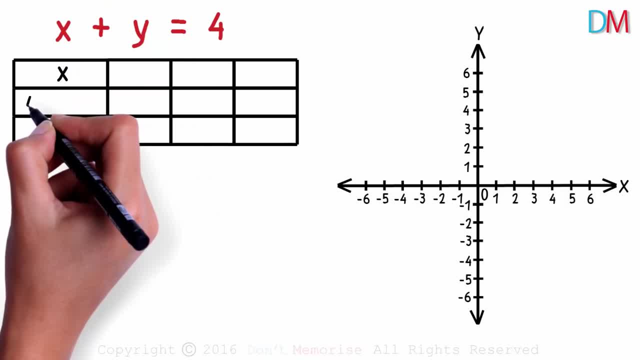 So let's make a table here that has X values in the first row and Y values in the second. Now let's take three random values of X, Say negative 1,, 0 and 1. And with these X values let's see what values. 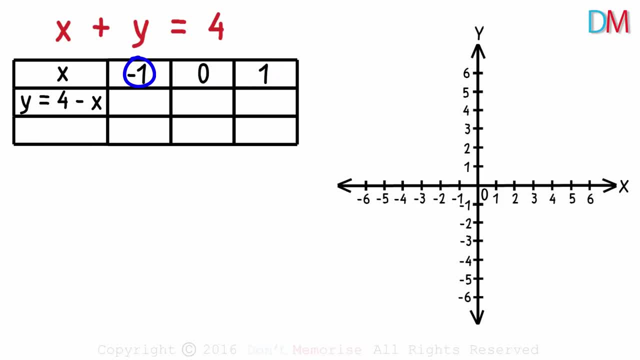 we get for Y. If X is negative 1, then Y will be 5. Because 4 minus negative 1 will give us 5.. If X is 0, then Y will be 4. And if X is 1, then Y will be 3.. 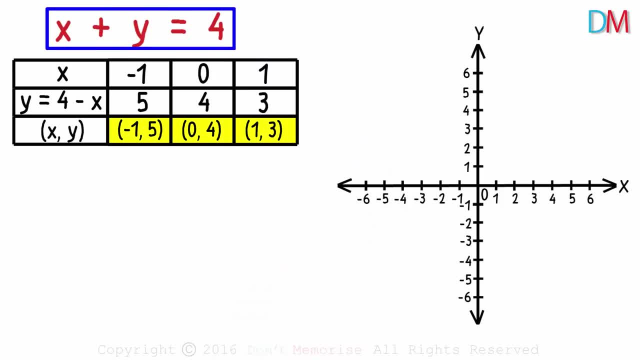 Now we got three pairs of values which satisfy this equation. Now, to get the graph of this equation, we just need to plot these points on the coordinate plane and join them. Negative- 1 comma 5 will lie here. 0 comma 4 will lie here. 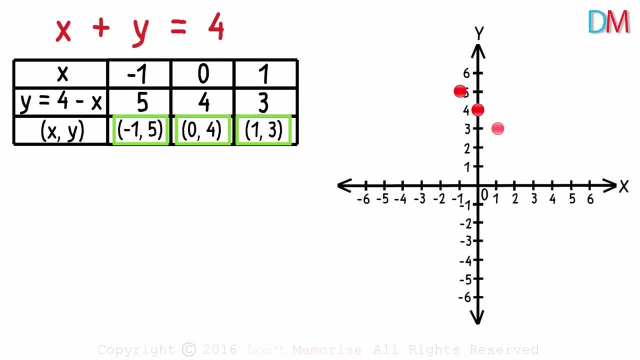 And 1 comma 3 can be plotted here. Now, when we join these three points, we will get the graph of this linear equation. On joining these points, we get a straight line. This is the graph of the linear equation: X plus Y equals 4.. 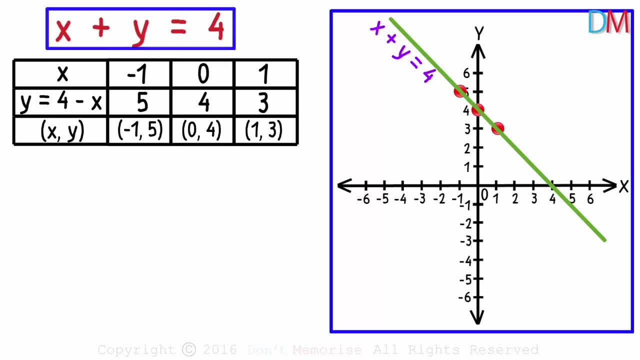 It looks like a simple graph, but there are many things we can infer from it. First, the graph is a straight line. The graph of a linear equation in two variables will always be a straight line. No matter what linear equation you pick, it's graph will always be a straight line. 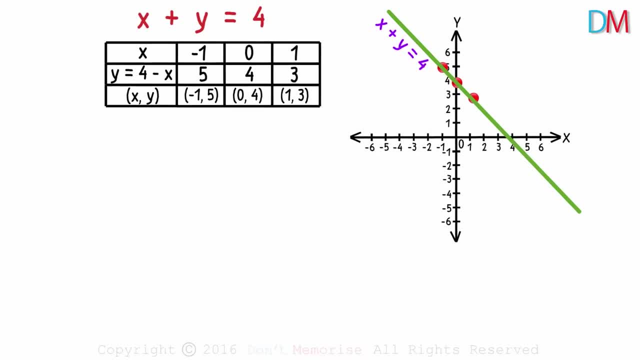 What else does this graph tells us? Another important thing it tells us is that whichever point you pick on this line, it will be a solution to this equation. Now, these three points we surely know are the relations of this linear equation. So now let's take another random point. 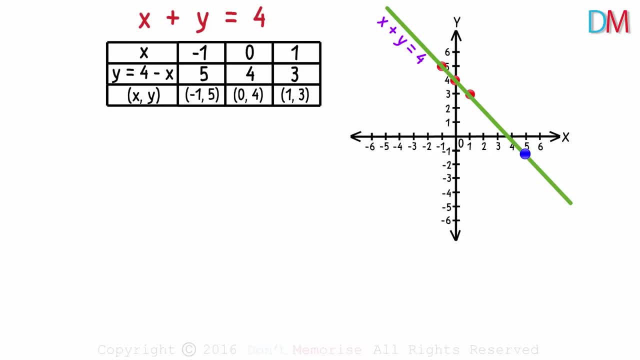 Say this point, It's 5 comma negative 1 when X is 5 and Y is negative 1.. Cold Done, You wasted our time, Let's do it quickly. 1, we see that the equation is satisfied. 5 plus negative 1 is 4..